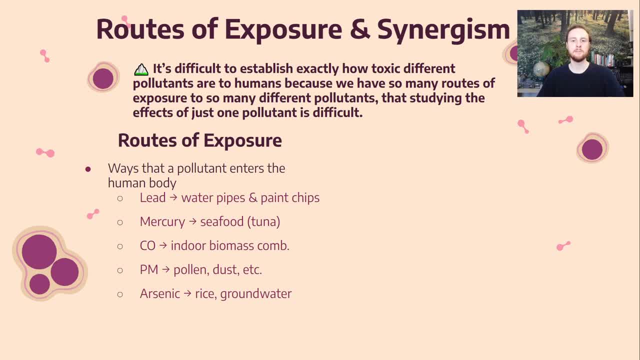 tuna, which comes primarily from indoor biomass combustion, especially in developing nations where subsistence fuels like charcoal or wood are heavily relied on and they're burned in open fires. indoors We have particulate matter, So anything like pollen or dust. this is just going to enter. 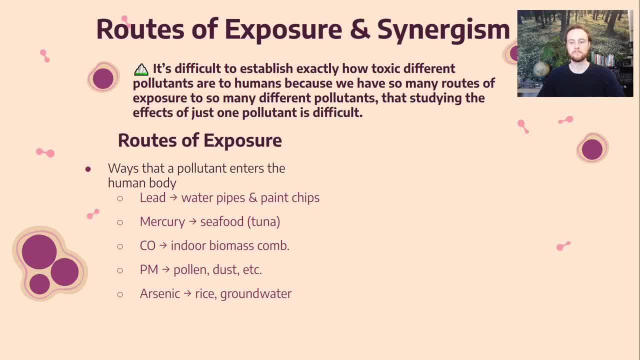 your respiratory tract just by virtue of it being in the air. We have arsenic, which can be exposed to the human body via rice. So sometimes rice will accumulate arsenic in its tissues And then when we eat it we take it into our bodies. but also groundwater that's been exposed to the air. So 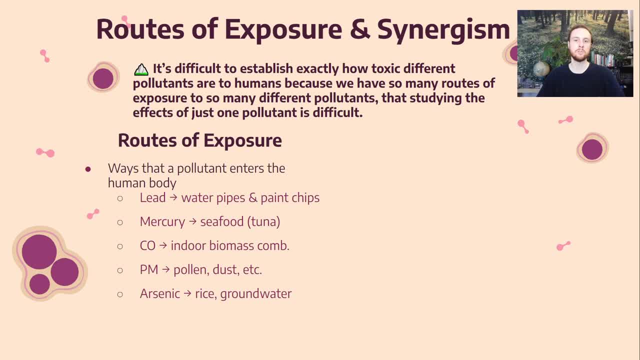 arsenic, either from you know, flame retardant chemicals or wood treating facilities that are releasing it, or just the natural decay of rocks that contain arsenic and releasing it into aquifers. Now we'll talk about synergism. So synergism is the idea that two or more pollutants or toxicants 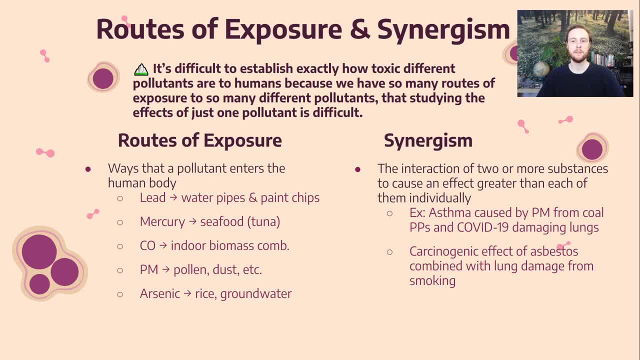 oftentimes have a combined effect on human health, or it could even just be an environmental condition, or what we have learned a lot about through COVID is pre-existing health conditions make a big difference to a patient's health, So if you're a patient, you're going to want to take a look at. 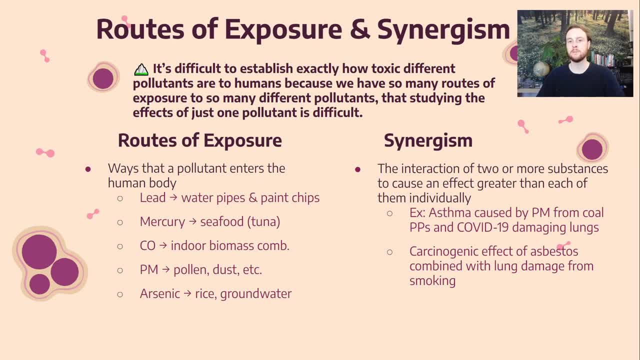 the pre-existing health conditions. So some examples of this would be the fact that asthma from particulate matter from a coal power plant could also be exacerbating COVID-19's damage to lungs. So it's hard to isolate the effect of COVID-19 when we could have an impact from coal. 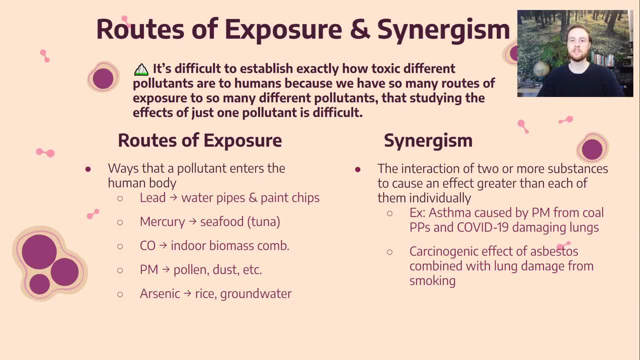 fired power plants nearby as well. Another example would be the carcinogenic effect of asbestos combined with the fact that someone was already a tobacco user or a cigarette smoker, So it's hard to isolate. is their lung cancer the result of asbestos, Or is it just the fact that they're? 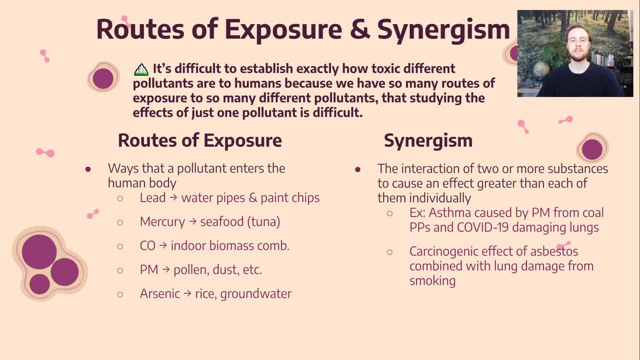 already a tobacco user, Or is it the result of damage from smoking cigarettes? And so this is this idea of synergism. Again, think of it as almost like a confounding variable. Really hard to look at a human and say your illness or your exposure to this toxicant is purely from this. 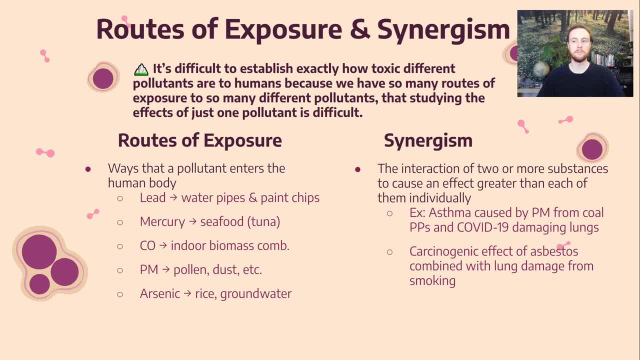 source And the cause of your disease or your condition is purely from this individual toxicant. So, again, it just makes it hard for epidemiologists to pinpoint the exact cause of an illness or disease. So even though we'll learn about some upcoming diseases that are linked to this, 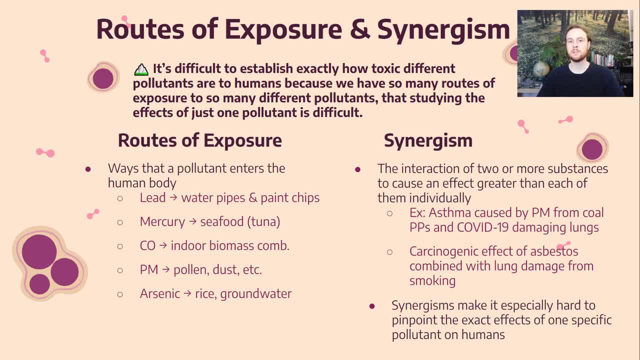 specific pollutants and toxicants. we need to remember that because humans are such complex organisms that do so many things in so many different ecosystems and environments, it's difficult to isolate the health conditions to one specific, you know toxicant. So the first human. 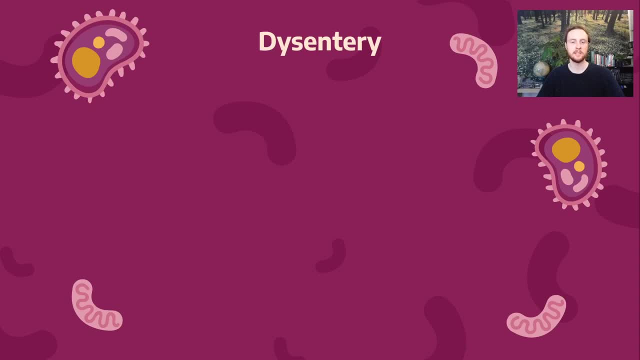 health disease that we'll talk about that is related to a specific contaminant or pollutant, is going to be dysentery. So dysentery is a bacterial infection that can occur in humans when their food or their water sources are exposed to raw, untreated sewage, And this is because that 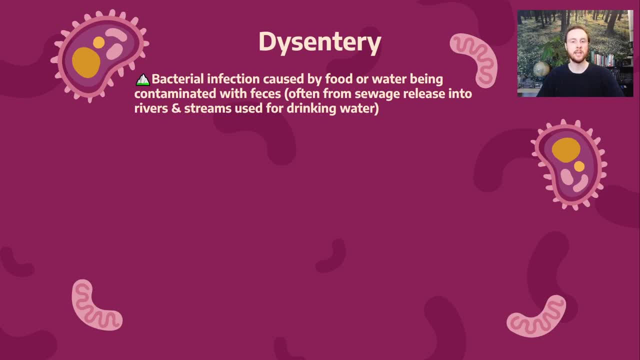 sewage contains feces. Now, this could be human feces, it could be animal feces, but this is really common in developing nations, where access to water treatment is not as widespread as it is in developed nations. So this is going to be a really deadly disease. It's going to cause 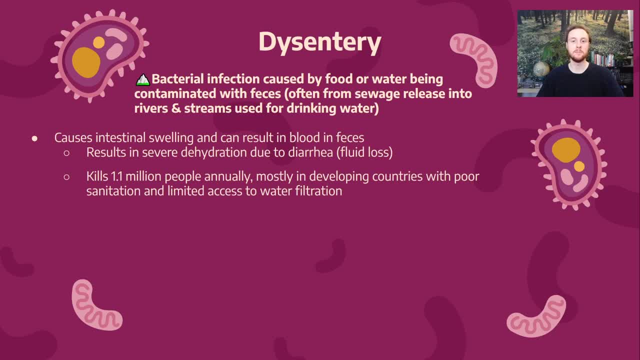 intestinal swelling. The bacteria will promote an inflamed- you know- immune system response and an infection that's going to cause potentially blood in the feces, in the stool. It can lead to really severe dehydration because individuals that have dysentery will oftentimes have really violent diarrhea And that's their body trying to flush that pathogen out of their intestinal system by just voiding the bowels constantly, And so it's a really problematic impact, especially for young children, because of dehydration. So their bodies are smaller, they're retaining less water And so, as a result, 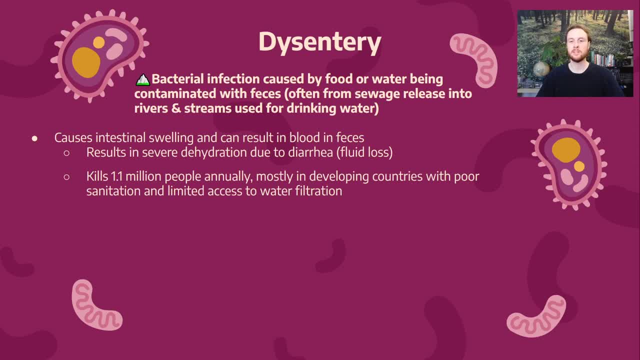 of this constant diarrhea. it can lead to dehydration. It's going to kill 1.1 million people annually, Again mostly in developing nations with poor sanitation where there's contamination of drinking water, especially with human sewage. So this is a really big problem globally And it's one of the reasons that so many philanthropists 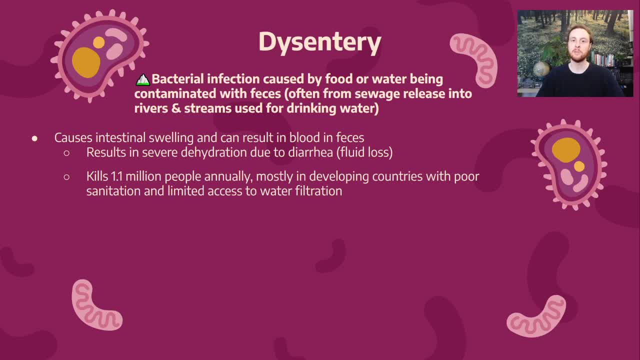 so many epidemiologists and environmental scientists that care about human health outcomes are focused on trying to expand clean water access filtration devices, And that's one of the main ways to prevent dysentery, Once a human has encountered dysentery and has been infected with. 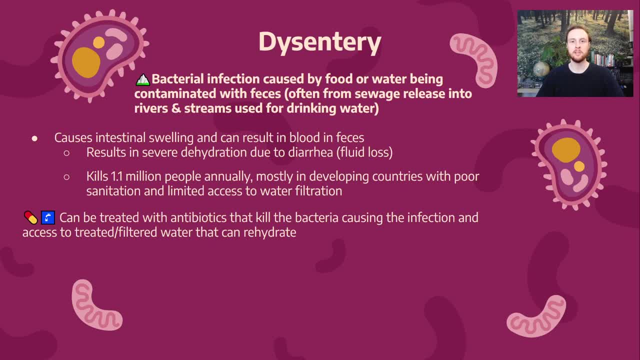 it. there are antibiotics that can be given to try to kill the bacteria And that's going to try to allow the body to stop having to again constantly flush the intestines out. So that can definitely help. Hydration can help as well If an individual is taking in, you know, a lot of water or liquids. 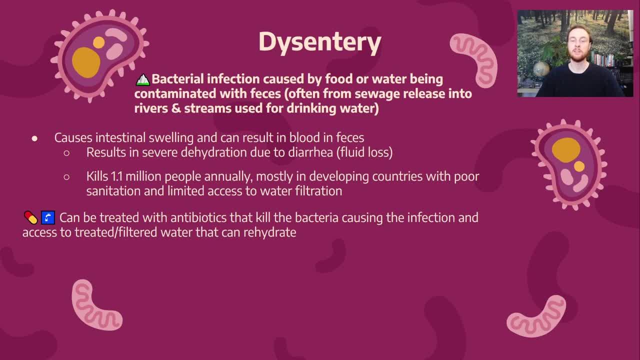 that have electrolytes that contain, you know, basically ions that help them contain and retain more water. that will help as well. And then, finally again, the way to prevent it is filtration of water sources, making sure that the water that people are drinking is clean. that is not. 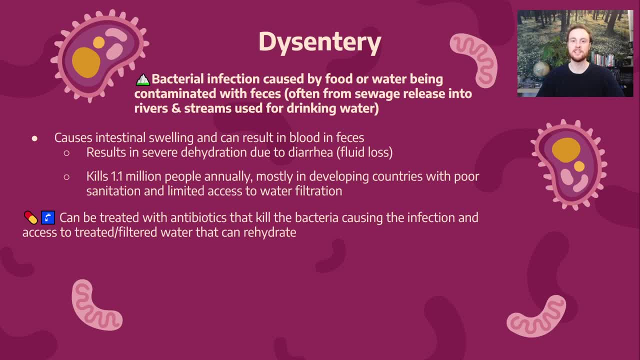 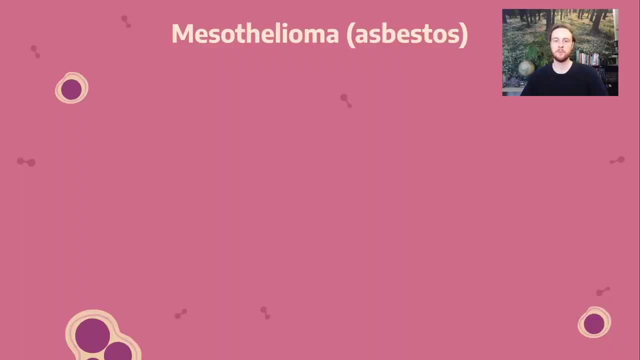 contaminated with the bacteria that cause dysentery dysentery and that it's not contaminated with dysentery and that it's not infected with human sewage. Next we'll talk about mesothelioma, which is a specific type of cancer that comes primarily from exposure to asbestos. 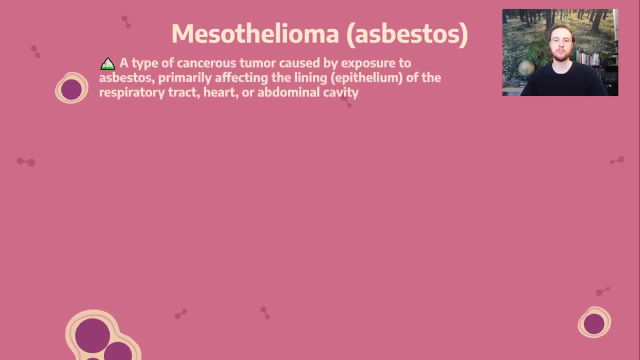 So when asbestos is exposed to the respiratory tract, when the particles are inhaled, oftentimes it will lead to the development of these cancerous tumors in the lining or the epithelium of things like the respiratory tract or the heart or the abdominal cavity. 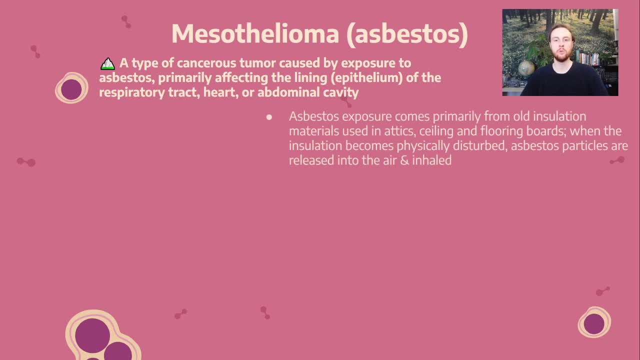 So what's the route of exposure here? Well, that's going to be primarily old insulation. So remember the water in the air istilated. So in the past we've used water to seal the toilet and the ceilings of buildings, sometimes even flooring tiles, or insulation used around water heaters. 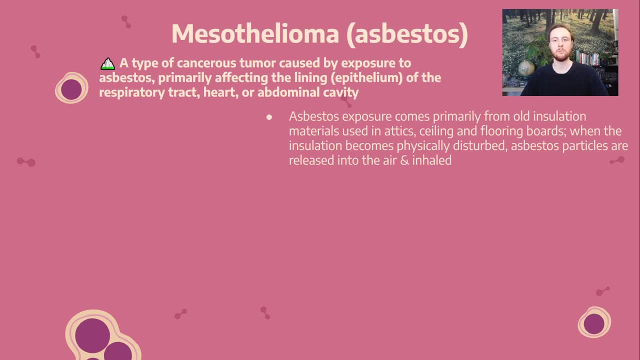 used to contain asbestos before we realized its carcinogenic effects, And so when those insulation sources are disturbed, when we go to renovate the area, if it's not done properly, those asbestos particles can make it into the air, they can be inhaled and they can have these. consequential effects on the human body. So we look here at the asbestos particles or fibers that are kind of being inhaled. They're going to turn. you know, this is like this. this is going to go like this. you know this. this will be somewhat glassy, but you're going to be able to see it. 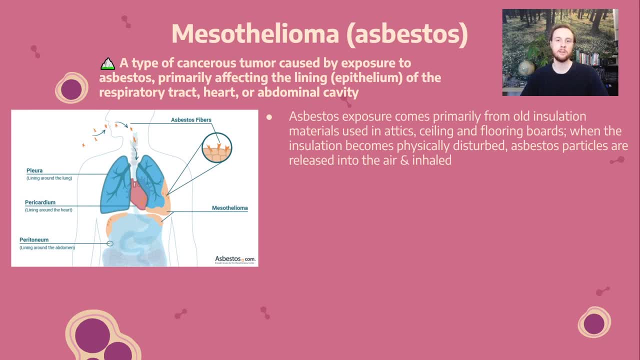 kind of being inhaled. they're going to target, you know, the pleura, the lining around the lungs. they can target even, you know, areas in the periosteum, which is basically the cavity in the thoracic cavity of someone. i'm just going to target the epithelium, the lining of these surfaces. 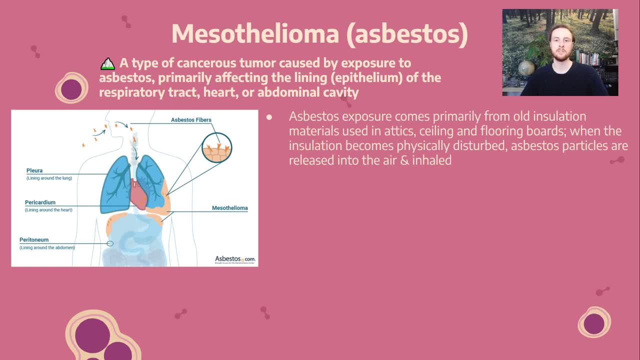 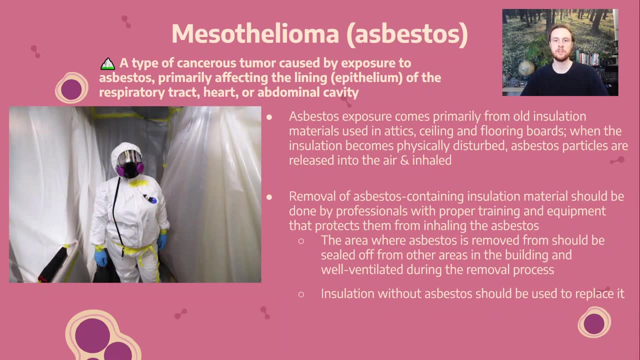 and it can lead to really problematic cancers that develop. so when we look at removal of asbestos, how should this be done? we want to be clear that it should be done by professionals who are wearing proper ventilated materials. they're going to have a respirator and a mask like this to keep it out. 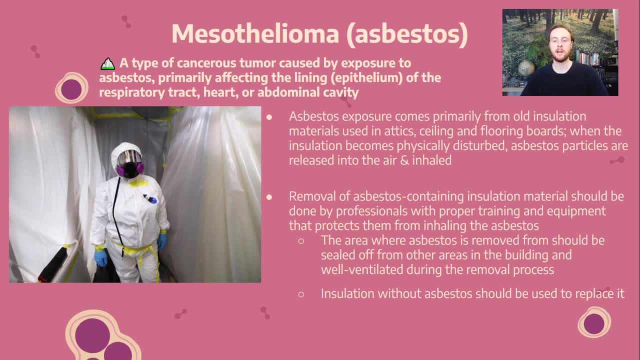 of their eyes to keep it out of their lungs. they're going to have a body suit that's going to keep it from getting attached to their clothing or making contact with their skin. notice that the area is completely sealed off, and so we're trying to prevent any asbestos. 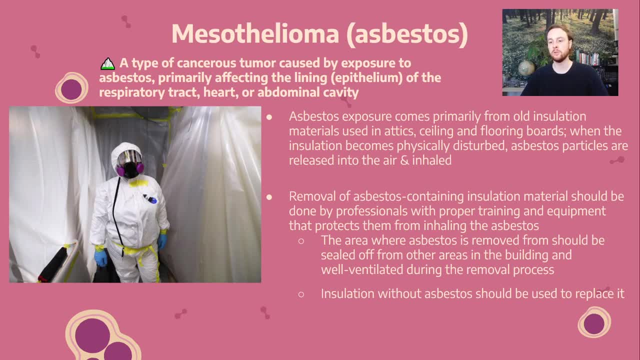 particles that enter the air from entering other parts of the building. you're going to want to have good ventilation. you're going to want the particles to be, you know, routed outside, where they can disperse and not build up Ishelm inside and be inhaled by the people that are doing this work or the people in other parts of the. 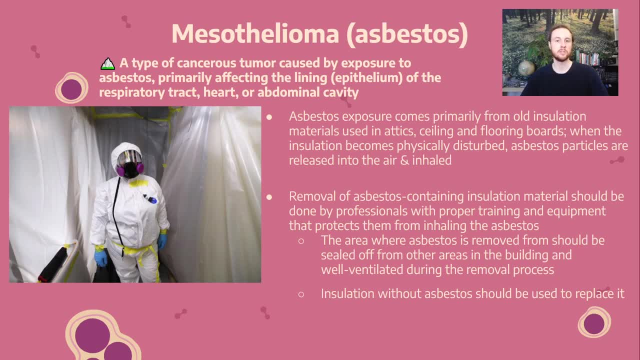 building. So I can't stress this enough. It needs to be done by a trained professional. You should not be removing asbestos containing materials yourself. It needs to be done by trained professionals. And then this may seem obvious, It may seem like it goes without saying, but if you 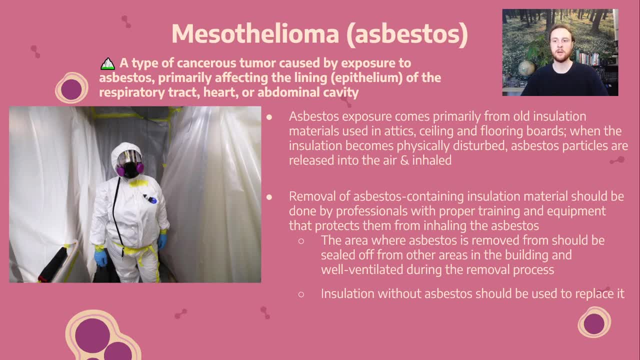 were writing an APES FRQ about asbestos and about reducing the threat of mesothelioma, you would really want to specify that the insulation that replaces asbestos should be asbestos free. I know that seems super obvious, but what I'm trying to do here is just point out FRQ writing skills that 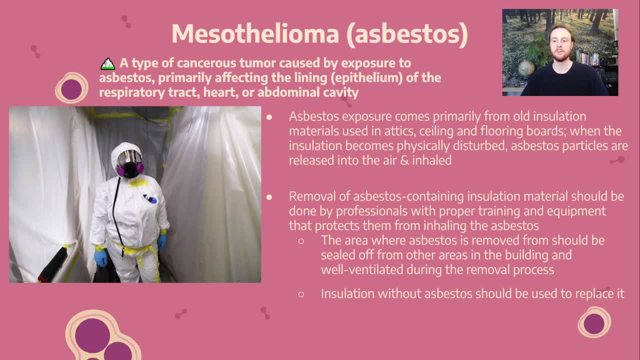 can, you know, elevate your answers and increase the likelihood that they earn points. So you really need to be clear that asbestos should be removed by professionals who are wearing equipment that allows them to breathe filtered air, not get the particles in their skin or on their clothing. 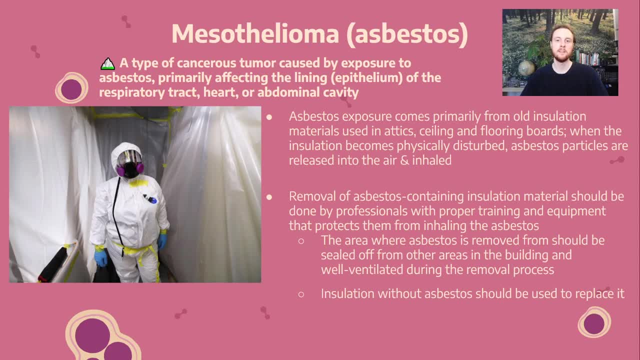 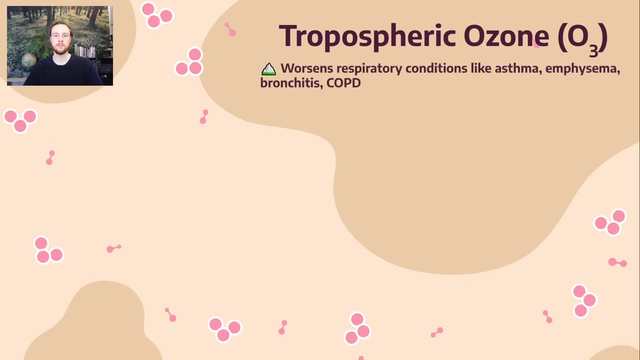 and that they should replace the insulation with non-asbestos containing materials. And we'll wrap up today by talking about tropospheric ozone. So remember that tropospheric ozone, or O3, is going to be a general respiratory irritant. So it's going. 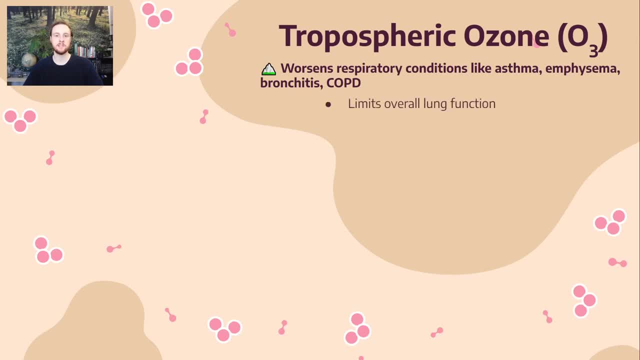 to decrease lung function. It's going to worsen pre-existing respiratory conditions like asthma, emphysema, bronchitis or COPD. So it's not so much that it gives you an acute lung disorder like this, but it's going to worsen your overall lung function and exacerbate or make worse. 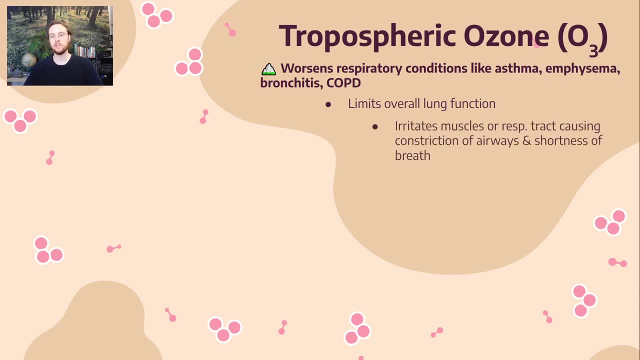 pre-existing respiratory conditions. It can also irritate basically the muscles of the respiratory tract. It can constrict the bronchioles or the air passageways that are bringing air into your lungs. So it can really have some dramatic consequences on the human. 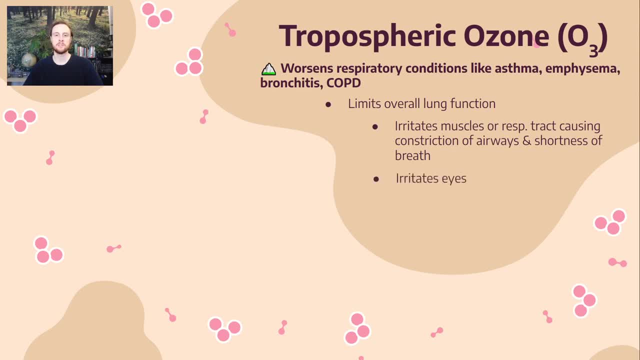 respiratory system. It can also irritate the eyes, So it's something that is really harmful for a variety of systems in the human body, but primarily the respiratory system. We take a look here at a diagram that can just help us kind of remember and visualize some of 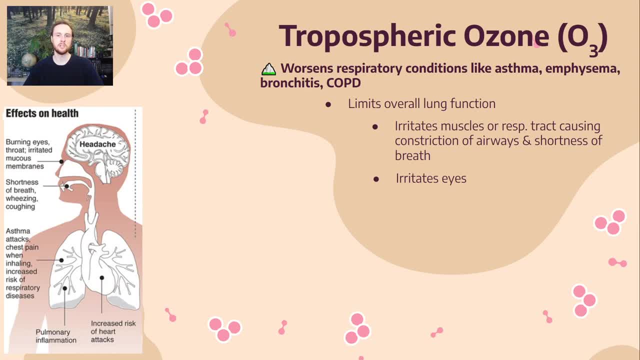 these. You know it can cause kind of a burning sensation and irritation of the muscles and the lining in the throat. It can result in a burning sensation and irritation of the muscles and the lining in the throat. It can result in a burning sensation and irritation of the muscles and the 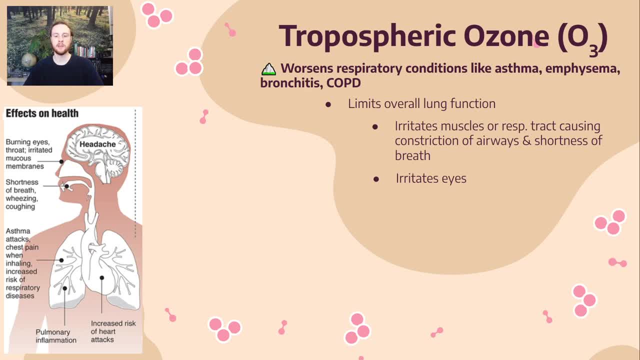 a pretty severe headache. It can be burning or irritating to the eyes And then, once it gets into the lungs, when it's inhaled deeper in the respiratory tract, you know, it can cause coughing. It can cause, basically, you know, acute attacks of asthma flare-ups. So really a problematic. 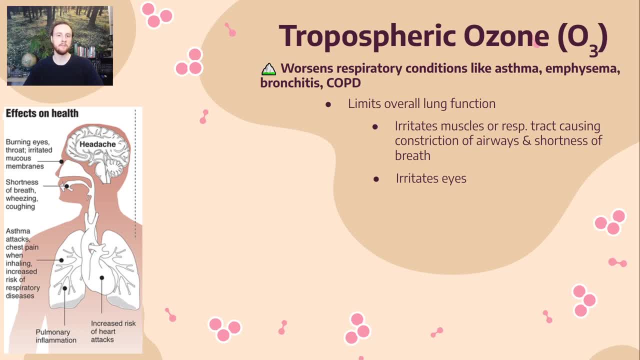 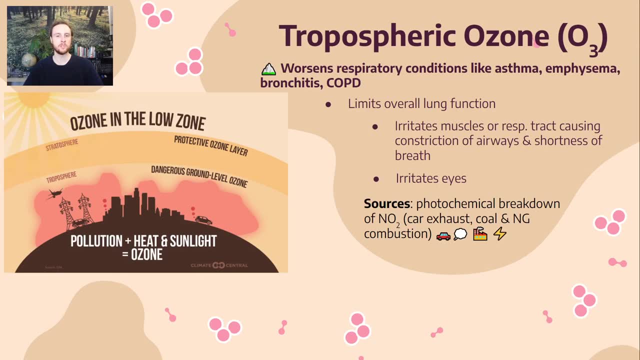 respiratory irritant in a variety of avenues here. So if we take a look at some of the sources of ozone or the routes of exposure, it's going to primarily come from NO2 emissions. Remember, the NO2- nitrogen dioxide- is going to be emitted from the lungs, So it's going to be emitted from the 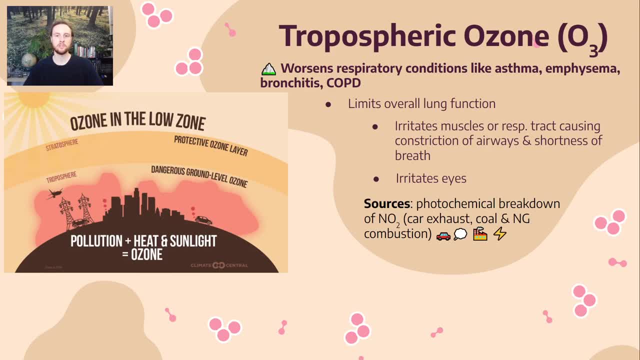 lungs. So it's going to be emitted from the lungs. So it's going to be emitted by vehicle exhaust, by coal-fired power plants especially, And it's going to combine with the sunlight And the sunlight's basically going to knock off one of the oxygen atoms from that, NO2.. That free oxygen atom. 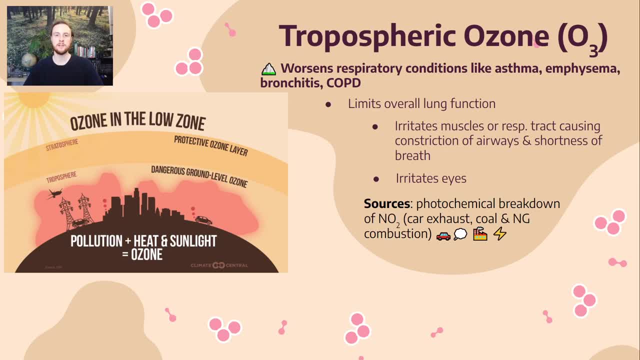 combines with O2, molecular oxygen in the atmosphere. Now we have O3 and that's ozone. So I've added a little edit here to this otherwise great diagram that I found online. It's not pollution plus heat and sunlight, It's NO2.. So not an apes-approved. 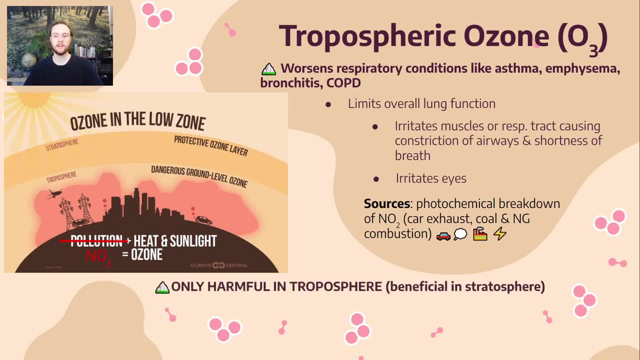 diagram without that little edit there. And then one final thing I want to recommend that we remember. really important is that ozone is tremendously beneficial when it's up in the stratosphere where it absorbs a lot of UV radiation that could be cancerous or cancer-causing for. 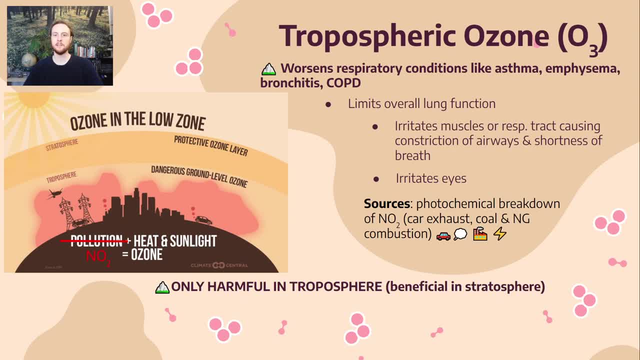 humans that can damage plant tissue. So in the stratosphere it is essential to life on earth. In the troposphere it's harmful And again, that's because of these respiratory irritating effects that it has. So if we take a look at the stratosphere, we have a lot of UV radiation. So if we take a look at the 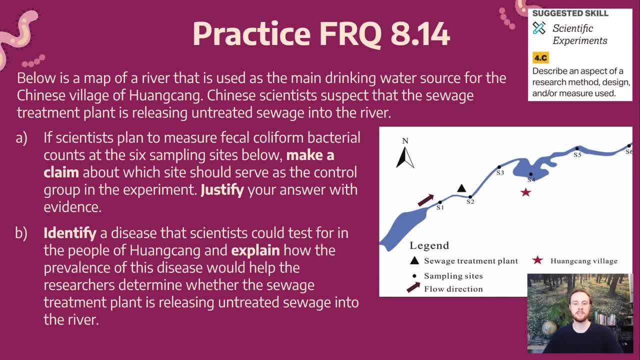 stratosphere we have a lot of UV radiation. So if we take a look at the stratosphere, we have a lot of UV radiation. So for FRQ 8.14: today we have a scientific investigation that we're going to look at. 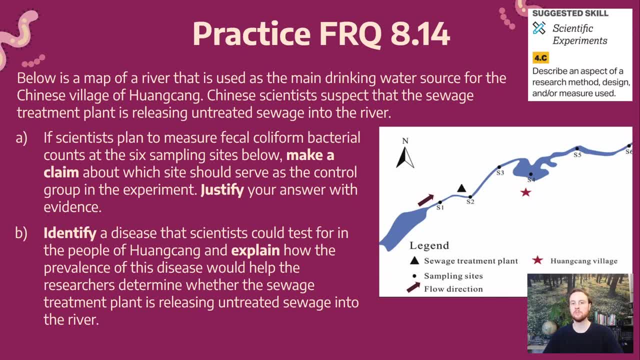 and we're going to try to come up with a claim about which groups should serve as the control and also a disease that these scientists could look for in the population of the people of Huangshan to basically see if this wastewater treatment plant that we can see in the triangle. 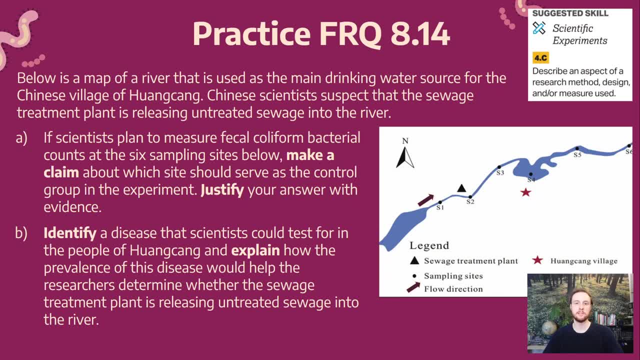 here is impacting their water quality and if it is leading to raw sewage being released into the river. A couple of things to point out. the flow of the river: So you want to look at the flow of the river. You want to look at the flow of the river, So you want to look at the flow of the river, So you want to look at the.